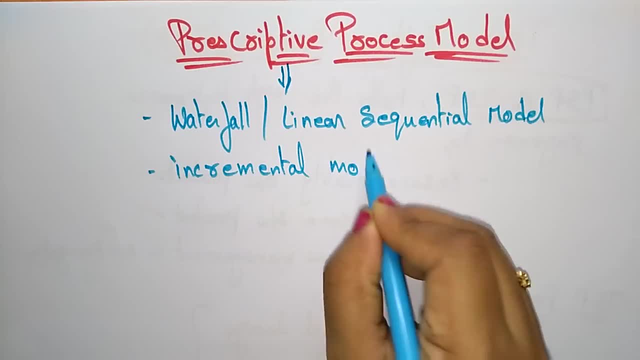 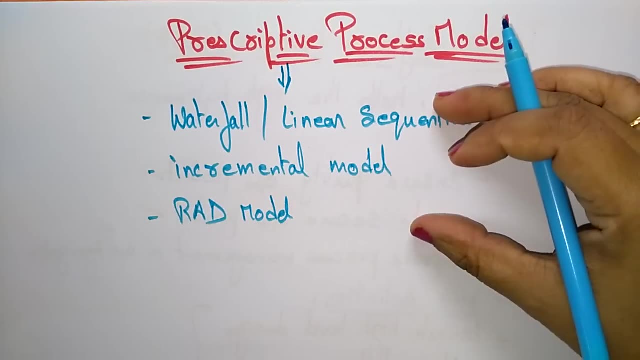 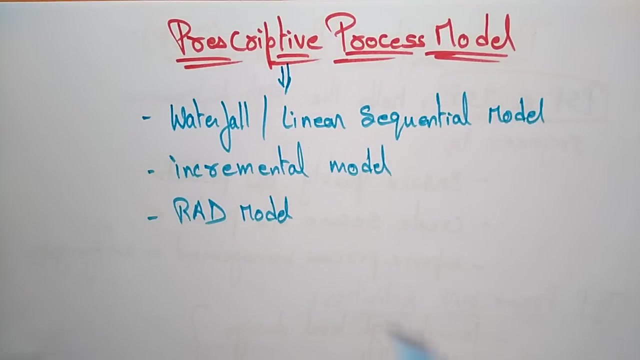 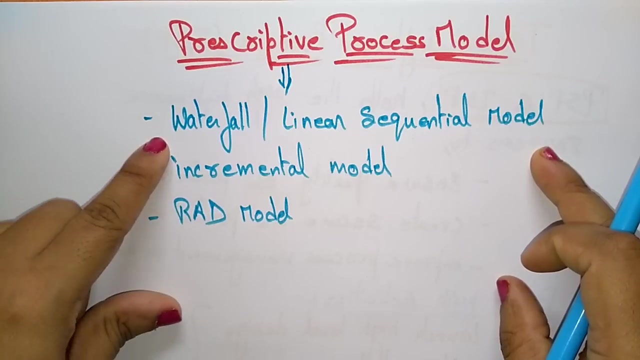 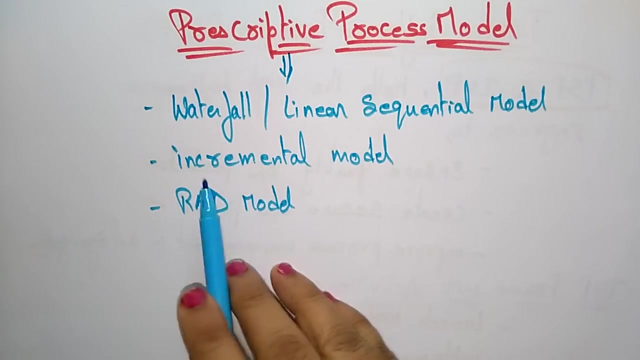 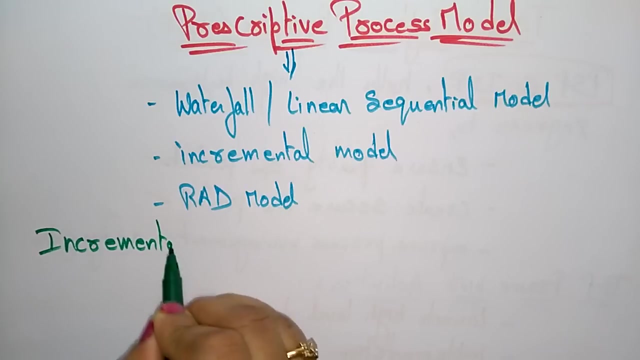 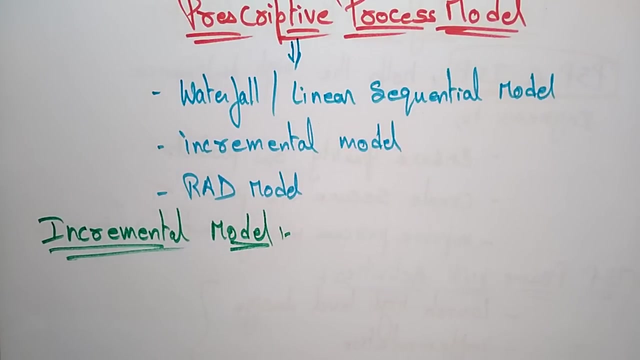 So what are the different types of prescriptive process model? Now let us see The different types of prescriptive process model are: waterfall model. we call it as also the linear sequential model. we call it as also the linear sequential model. Now let us see the next. that is an incremental model. Now let us see incremental model. So, incremental model? actually, it is used when requirements are well understood. Whenever you are the person, the person who is implementing the project, the team that is going to implement the project, they have to well understood the requirements, whatever the requirements are. 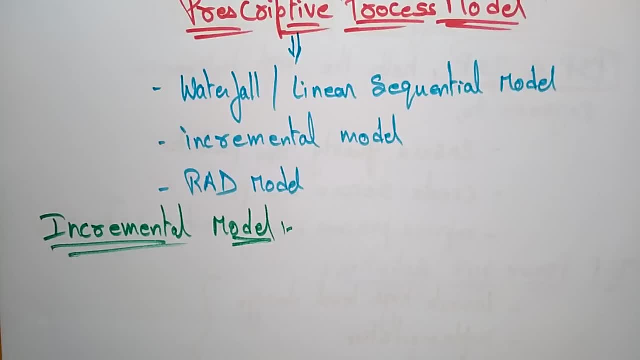 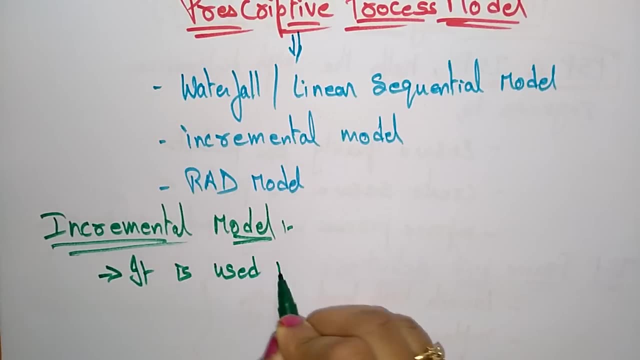 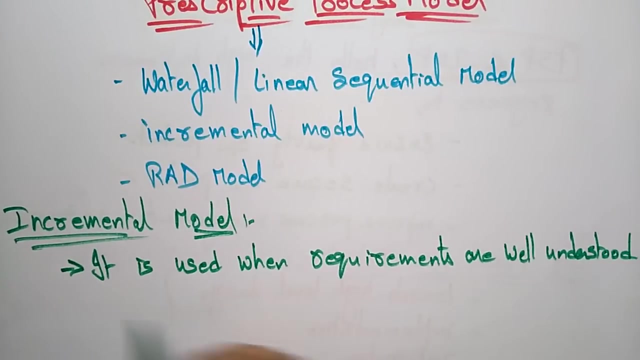 in the incremental model. So let me write the points. first, Incremental model. it is used when requirements are well understood. then only you proceed with the incremental model. The next point: Multimultiple Independent Deliveries are identified In incremental model. 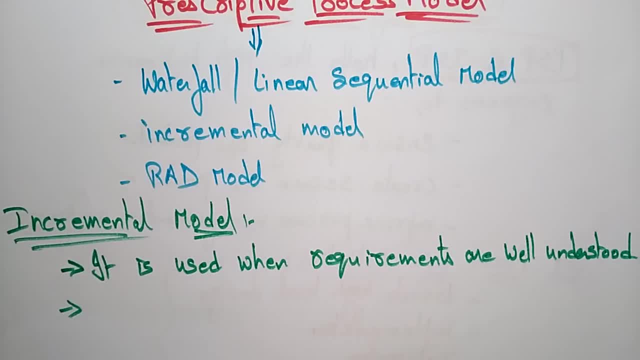 you will think to. Я came across you will under identify the multiple independent deliveries means once one module is over, means one concept or one module is completed, then the delivery will be there and the multiple everyone is independent to the other. okay, it's a small unit- modules, so every module will be. 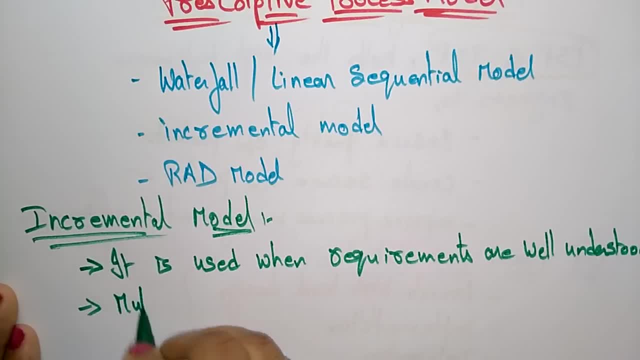 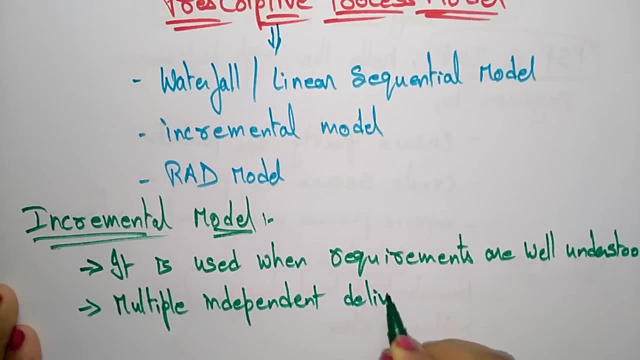 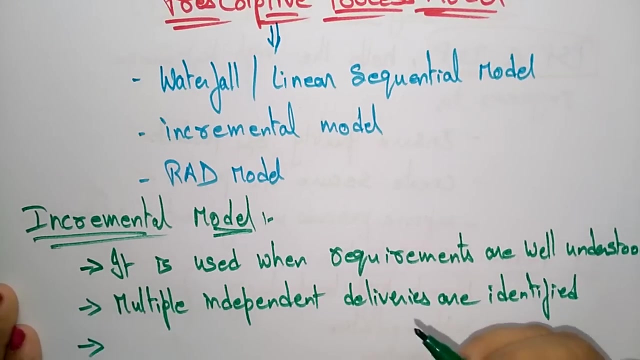 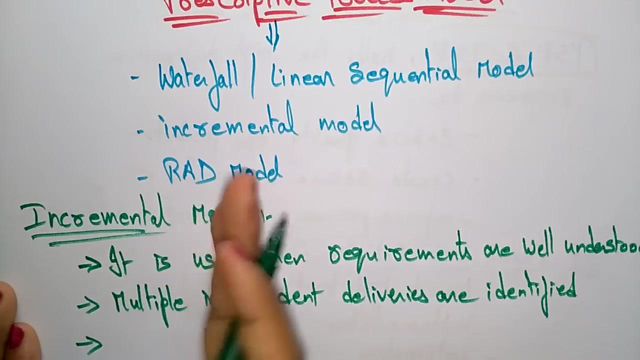 delivered independently, multiple independent deliveries or identified in the incremental model. and the next point: here the workflow is linear fashion. so just like a waterfall model, the incremental model is also. the workflow is linear fashion within an increment and staggered between an increment. so within an increment and in the 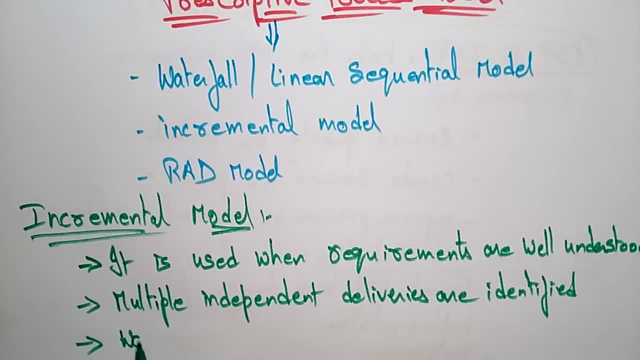 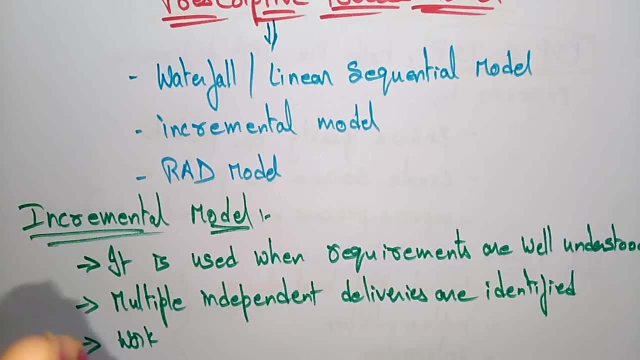 staggered between the increment. the workflow is always linear. means after the completion of communication they go for planning. after the completion of planning they go for modeling, like that: after the completion of one phase only, they will shift through the another phase. once that that phase is freezed then goes to the end of phase, like that. so it's. 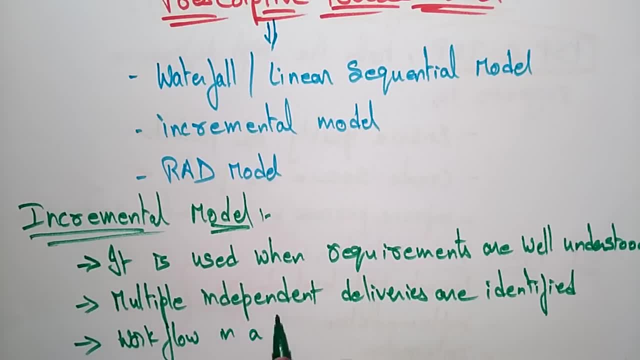 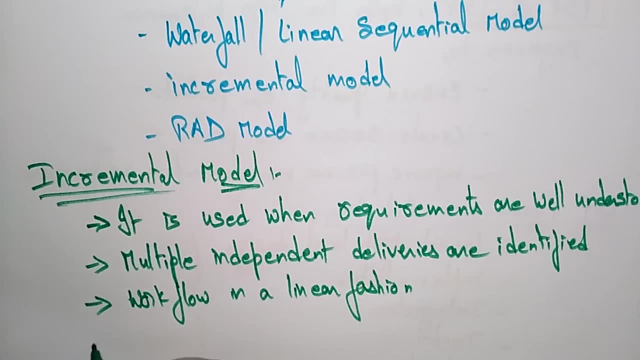 a sequential flow, work flow in a linear fashion, in incremental model, and here the it. uh, the concept of iterative will become incremental model also. uh, the iterative will become means once planning is over again, they try to communicate with the person. is still any requirements on there like that? so it is iterative in nature. 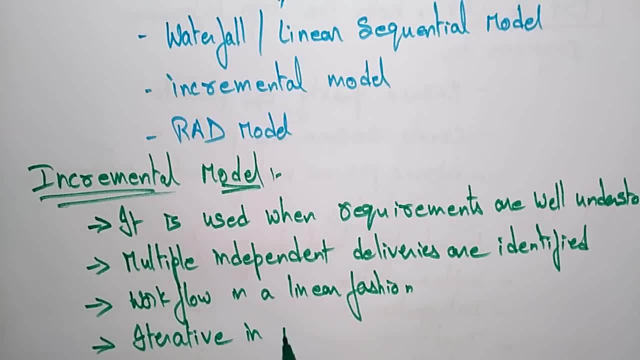 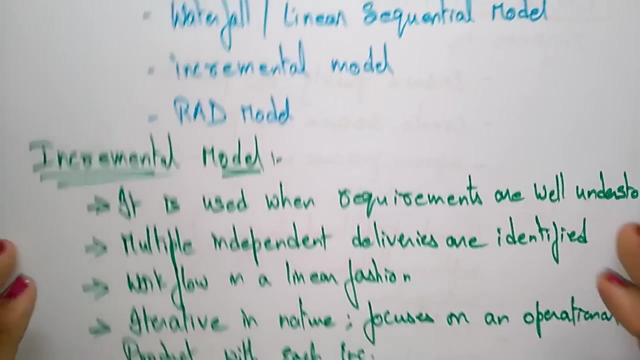 iterate you in nature and it focuses on an operational product with each increment. it focuses on an operational product with each increment. so this is about the incremental model. so it is used when requirements on each p model it very time so that just cinco much like a long time action split. meantime it use ап. 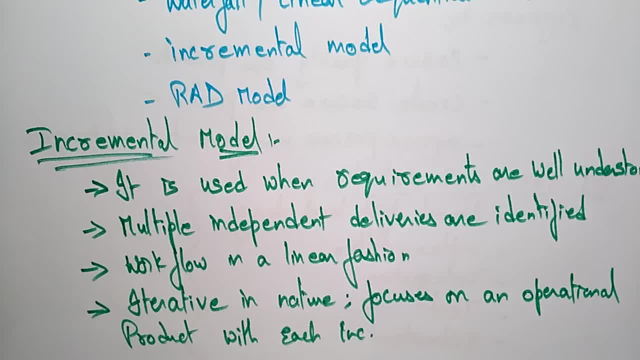 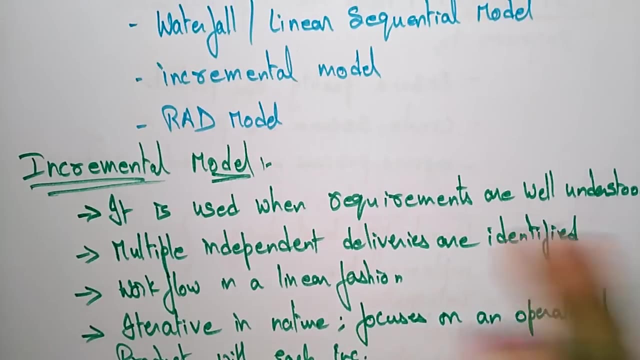 or well understood. then whenever there is a multiple, i mean it is a concept of delivering the multiple independent modules. so the multiple independent deliveries are identified in incremental model. here the workflow should be a linear, so that's why we are calling it as a prescriptive process. the prescriptive process always follows the sequential flow, the linear fashion, and 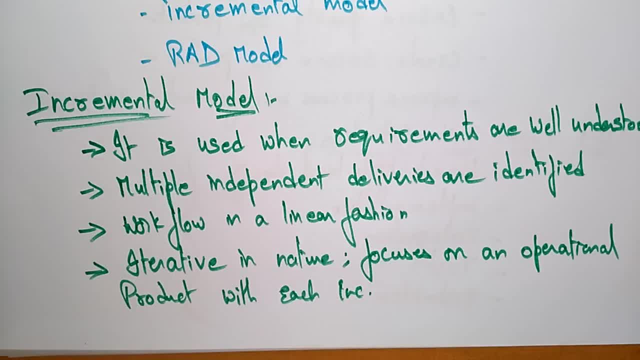 actually it should be iterative in nature. even though it is iterative in nature, but it follows the linear fashion, one after the other. okay, so in any stage some any problem is occurred, it should follow the iterative in nature and it is focused on an operational product with each increment. so 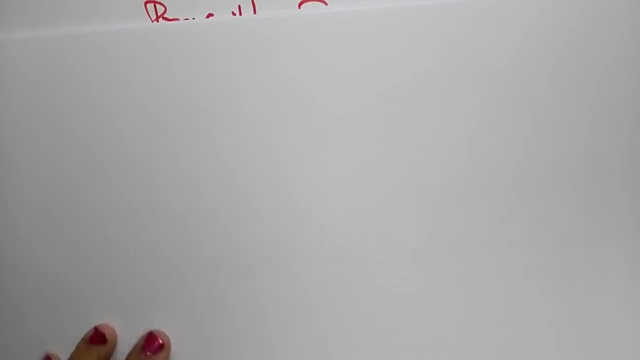 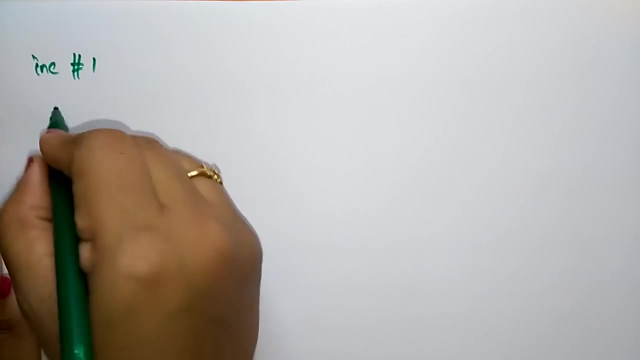 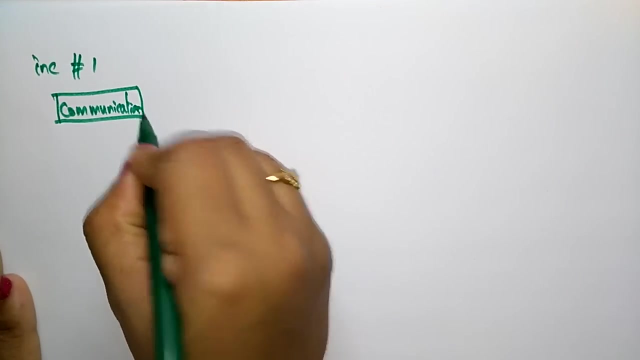 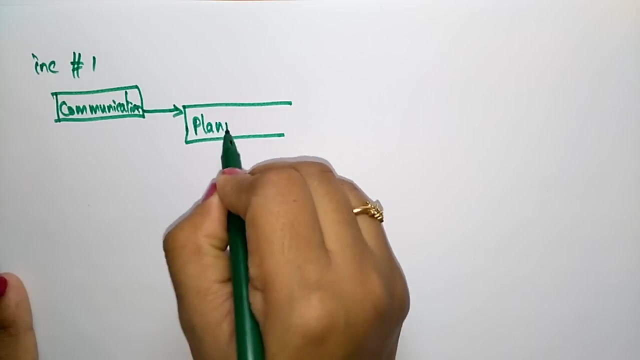 let me show you the diagram how this incremental model will be. let us take the first increment. this is one module increment one. so in the increment one they'll try to first communication, communication with the you customer. next they try to planning on the requirements. next stage is the planning. 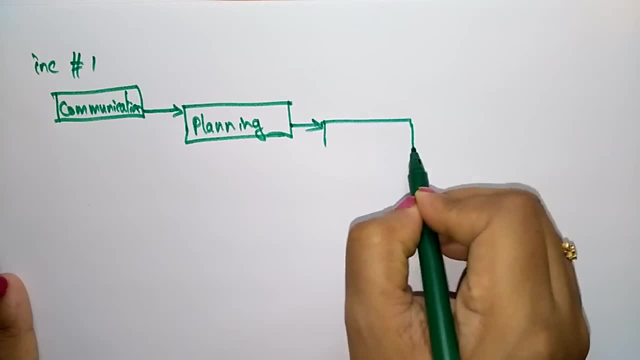 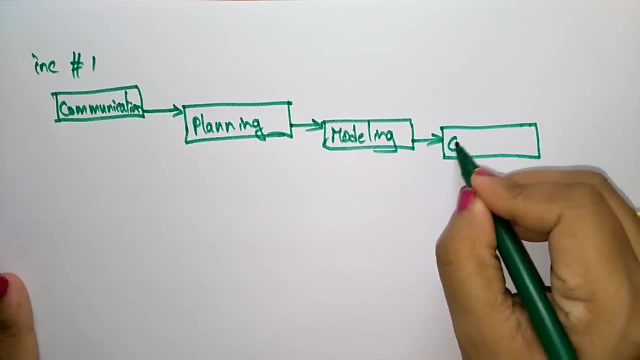 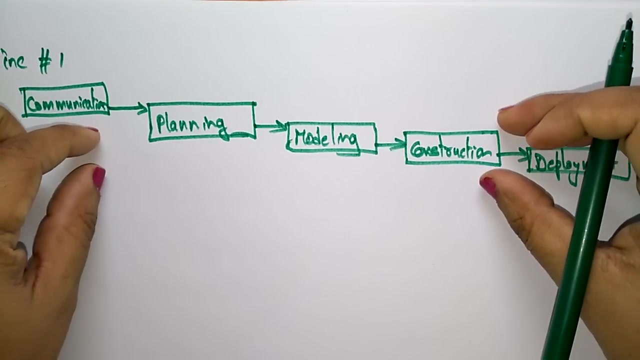 next stages: modeling. so after modeling they try to construct the product. means in implementation: construction, so final deployment. so once one module is completed, one iteration is completed. so they try to construct the product. so after modeling they try to construct the product completed, they try to deliver the product. so this is one independent process and next they'll take 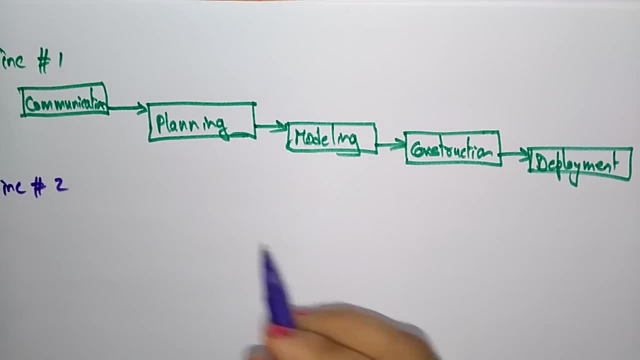 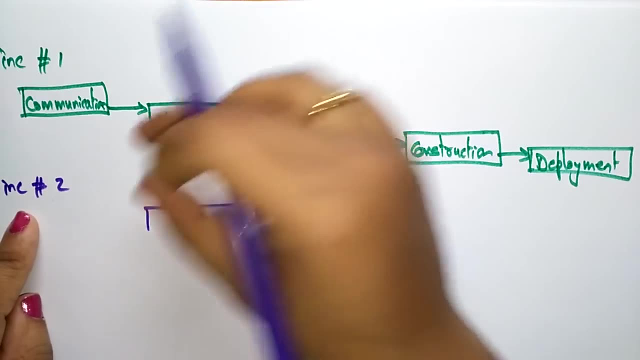 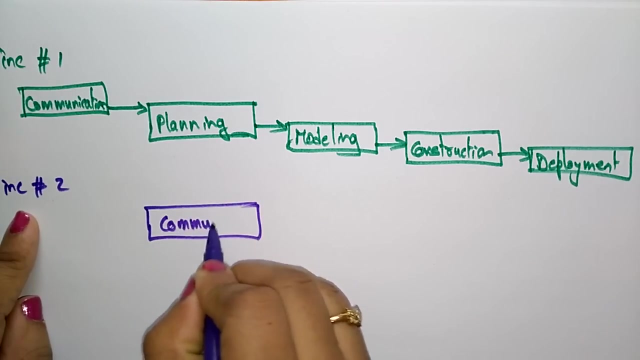 the another in increment two. so in the increment two they start with the. so once one one module is try to planning, do the work, so the another team will take the another module. they start with the communication with the first customer. they communicate with the customer, then they try to. 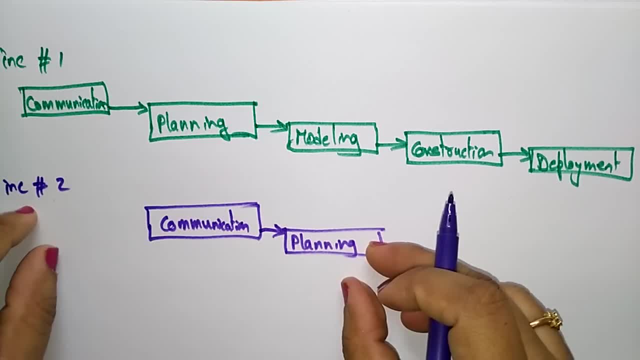 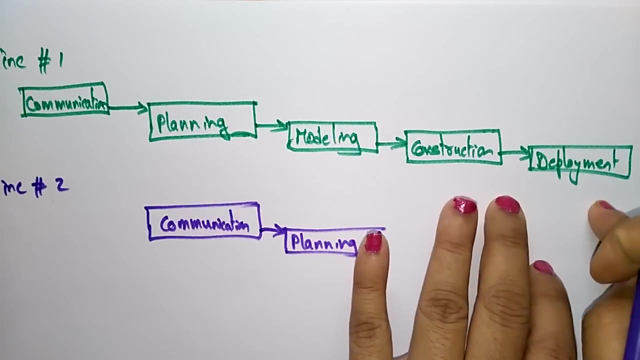 plan the project of the second module when this tea, this team is in planning stage and the first team be in modeling stage, because everything will be independent to each other. so there is no communication, there is no dependent relationship. so this will be, once communicated, if the product is successful, they can deploy and another team 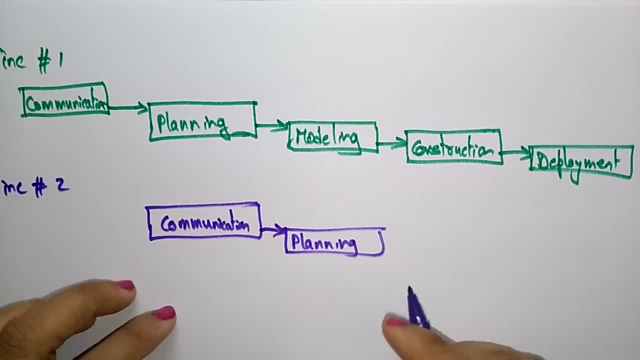 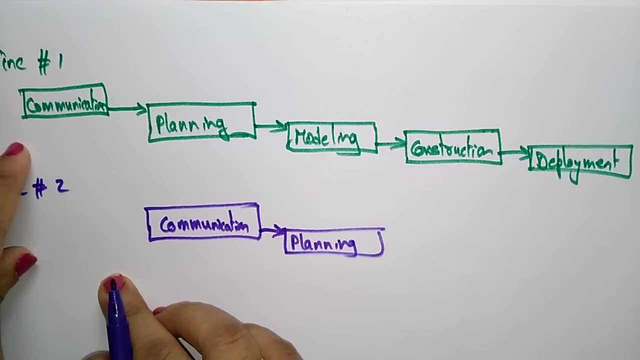 will take another module and try to communicate. so why we are starting? we can start here also. but the problem is if the same customer is there. if once the one customer is discussing with one module, once he hand over the project, then he'll take the another module and communicate with the people, so one team is in. 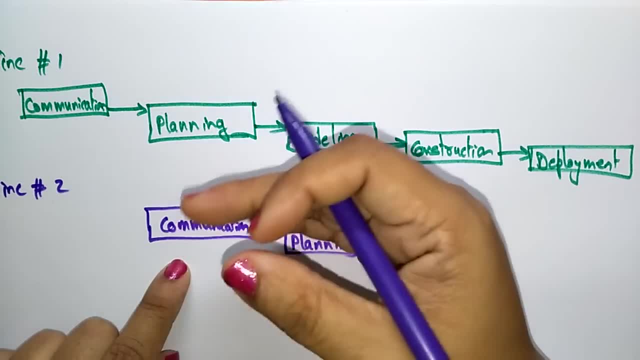 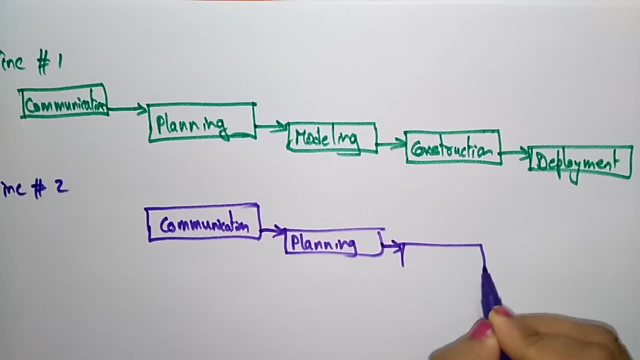 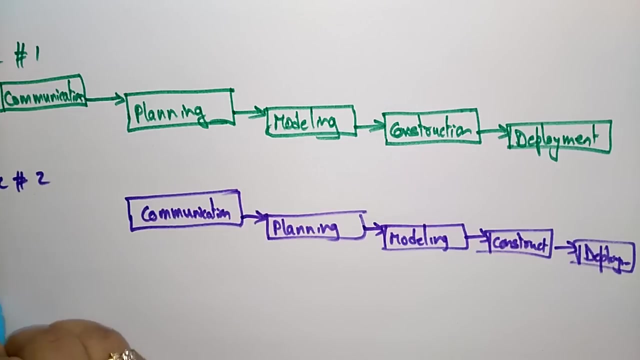 planning stage and another team will come to in the queue. okay, one after the another, so it is an incremental model, one after the another. so planning next, modeling next, try to construct and deploy. okay, so in another stage, in the increment three, so when they are in planning. 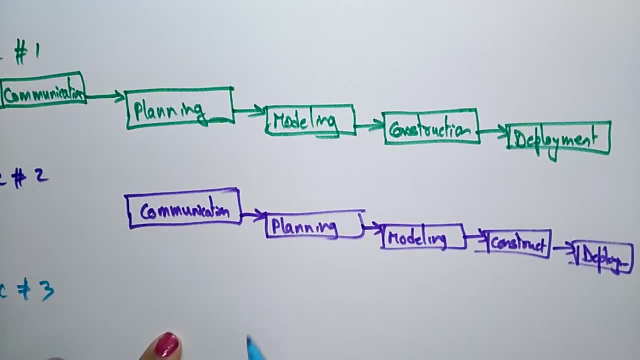 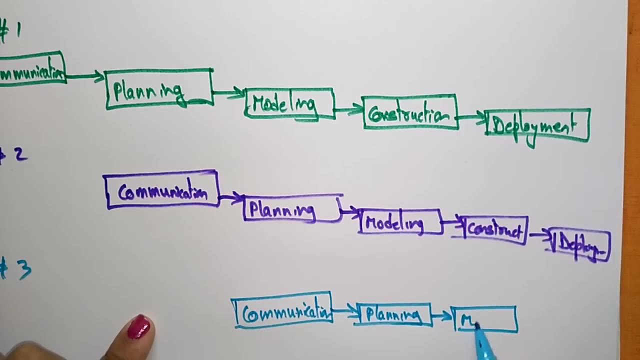 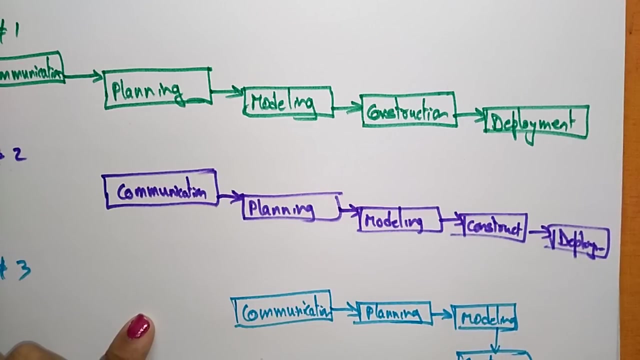 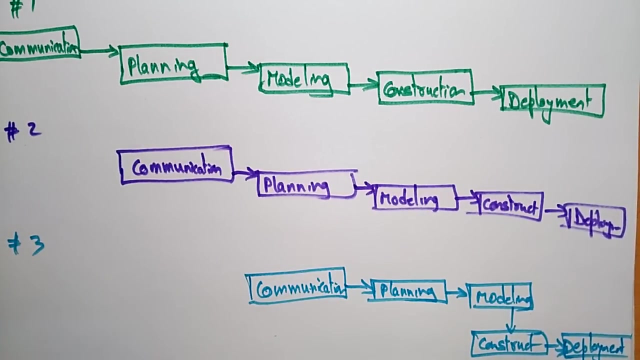 if one team is in modeling stage and next is in planning stage and and the third they are trying to communicate, communication, communication, next they are planning that module and modeling, next try to construct and deployment. so this is how the incremental model will be work, thank you,